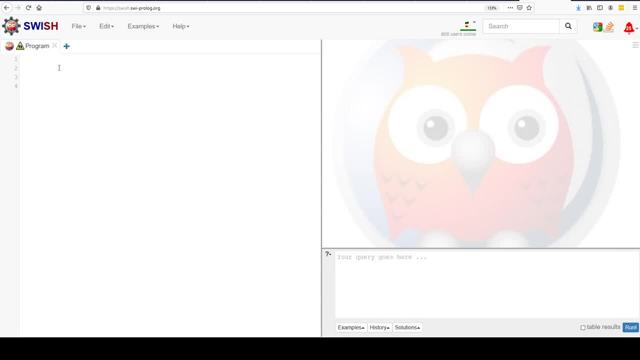 So if you're checking if an element is a member of a list or not, we need to be able to build a recursive function for that, because we need to be able to go through the whole list And in Prolog there's no loop. Instead, we have to use recursion. 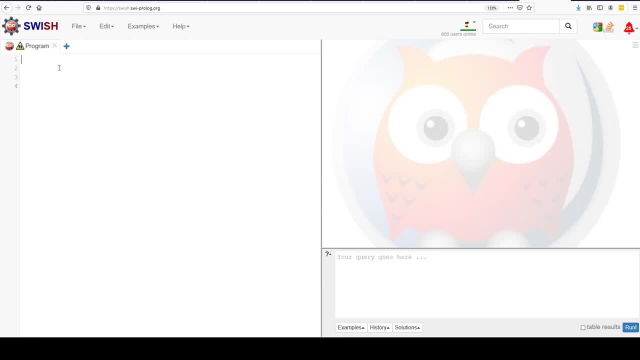 So, to start with any recursive or basically with any recursive method that you write, you're going to want a base case and then at least one recursive case. So the base case is where you should always start, And what you want to think about is: what is the? 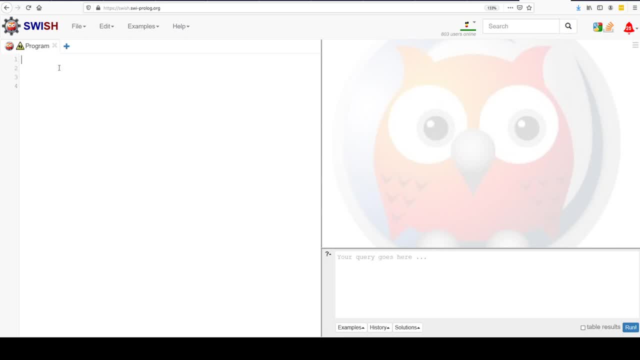 easiest way for me to be able to guarantee that I can return true for this problem, given the constraints of Prolog And specifically with lists. the constraint is with breaking a list into a head and a tail. what's the easiest way to verify? 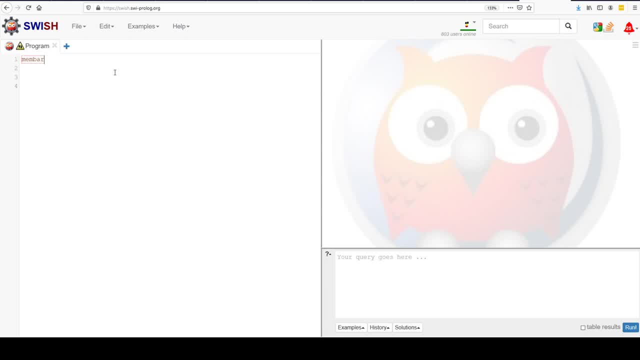 So the easiest way to verify is to check that an element is a member of a list. So let's set member and let's say that the element we're looking for is x, And so we're going to have the element we're looking for as the first argument here. The second argument: 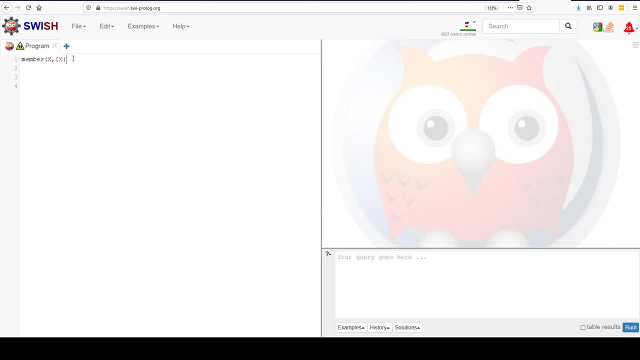 we're going to be given a list, So this is the list we're checking for that element in. If we split this list into its head and tail, the easiest way to verify is to check that an element x is in a list is if it's at the head of a list. If I can split a list, 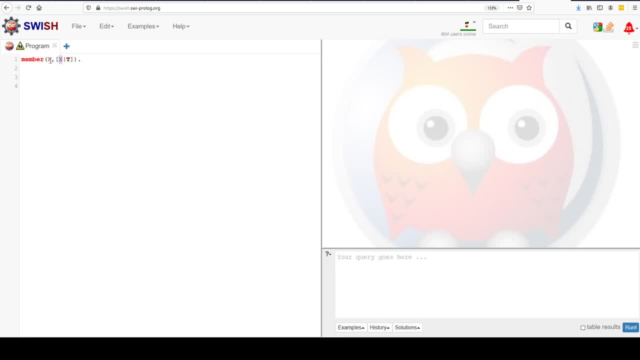 into a head and tail and the item that I find at the head of the list is the same as the item I'm looking for. well, that's easy, that's great. That's like saying we're looking for member Yolanda in the list. Yolanda Mia Vincent Marcellus. 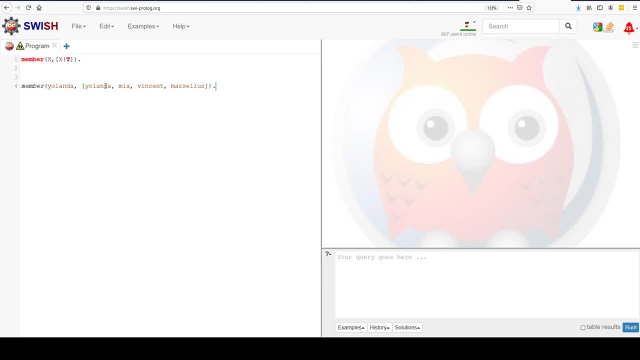 Well, this is our easiest case, because when we're working with lists, we always split into a head and a tail, And so if we split this list into a head and a tail, we're going to find Yolanda at the head and it's going to match, and we'll be in a really good place. 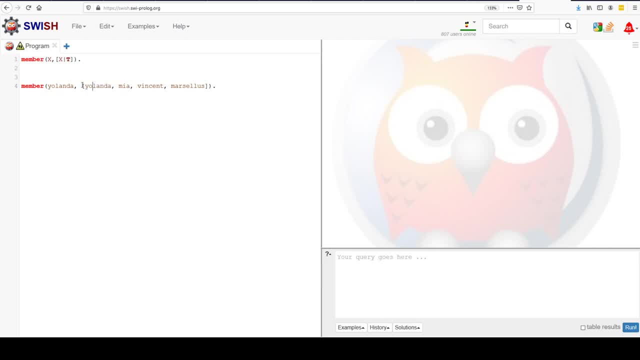 So the alternative here, the thing that is a little bit more tricky, is when Yolanda is a little bit further down the list. So let's say, instead of being at the head of the list, she was down here. Well, when we split this list into its head and tail, the head is going to be Mia and 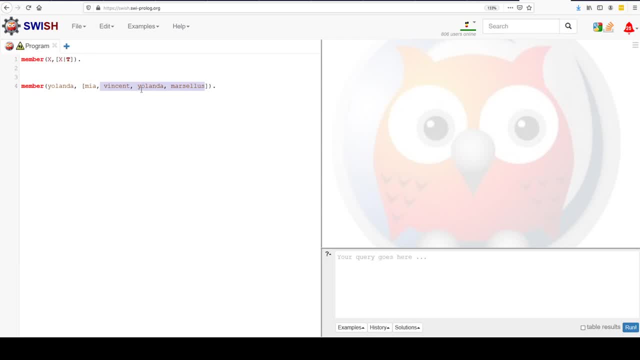 the tail is going to be this list of Vincent, Yolanda, Marcellus. So Mia and Yolanda don't match, so we're going to need to iterate again on the tail of the list check if Vincent and Yolanda are the same, which is what this predicate will do. If they are not, we need 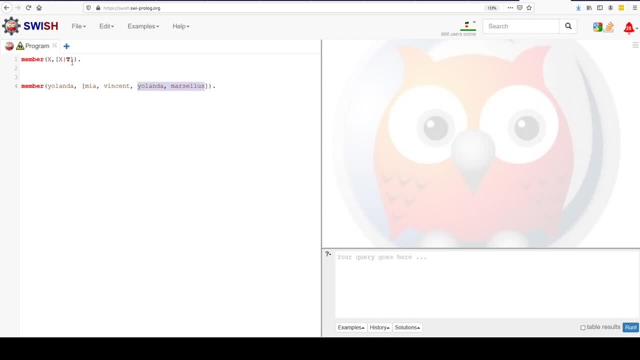 to iterate again and split the remainder of the list into a head and a tail, And then, in this case, we would finally hit our base case, where Yolanda, it would be at the head of the list. So as we iterate, 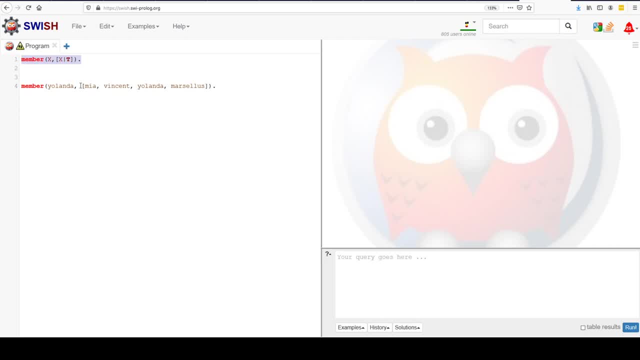 through. what we're really trying to do is just split the list into a head and a tail and feed the tail back in to try again. So what we need to be able to accomplish that is another member predicate that takes x and really importantly, here I'm going to stop before I write the rest of this notice. 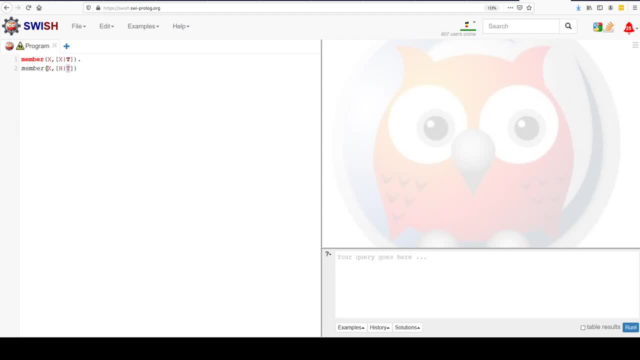 that we have h and t, not x and t. so we're going to have h and t, not x and t. so we're going to have h and t. If we put x here, we're basically checking the same thing. The item. 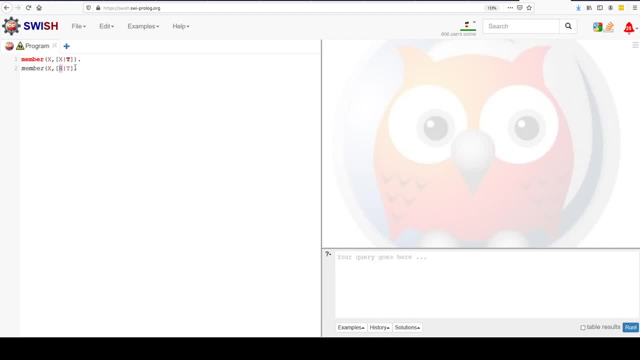 we're looking for would have to be at the head of our list. If we give them different variables, different variable names- x and h- then these are no longer required to be the same Right. so this is the case, for if they are the same- and this will be the case- 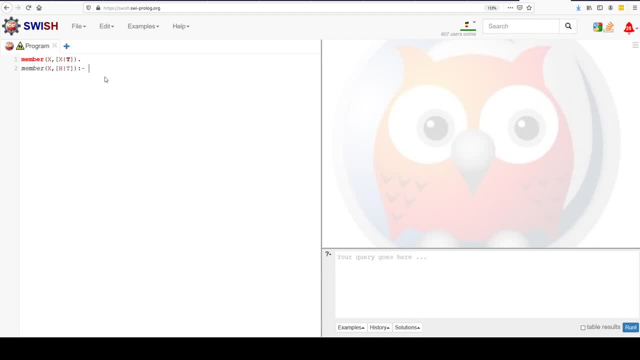 for if they are not the same. So if the member we're looking for and the head of our list are not the same, we need to recursively call member and we're going to call the head of our list recursively call member, given the same element we're looking for. so we want. 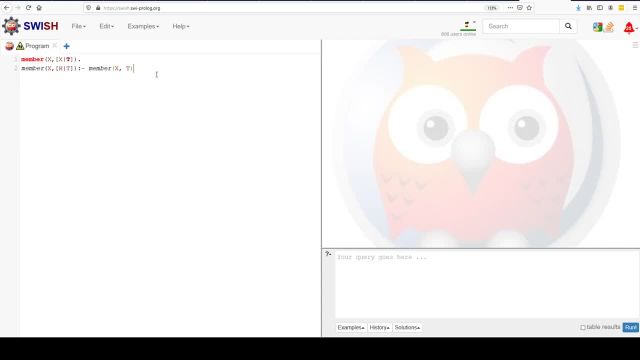 to pass that along to the recursive call and we want to pass the tail of the list to our recursive call. So the idea here is: we take a list, we look at our list. we're going to go through our predicates, first this one and then this one. We look at a list if the 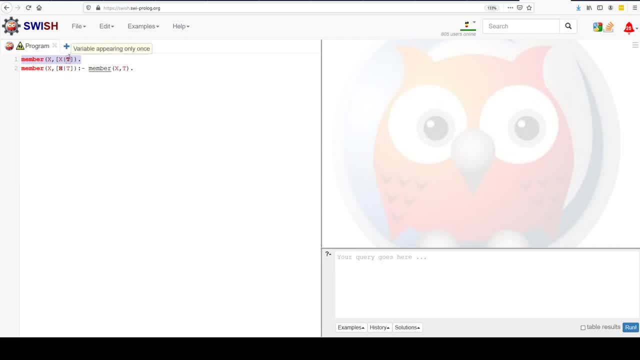 head of the list is the same as the thing we're looking for, then we return true and we're done. If the head of the list is not the same as the thing we're looking for- these are two different variable names- then we're going to call member again with the same element. 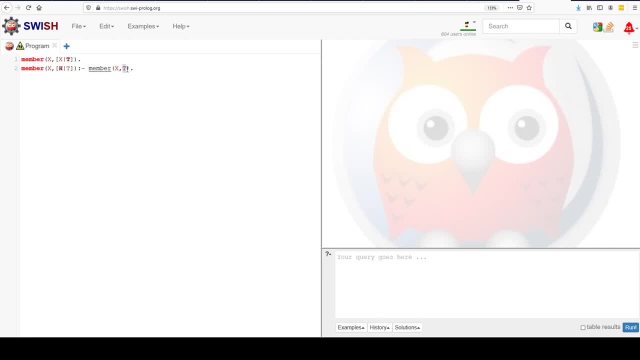 we're looking for right, we're still looking for the same thing, but now we're looking for it in the tail of that list, And so if you follow this pattern recursively- and we'll walk through an example here- you'll see how this will end up, finding every possible this. 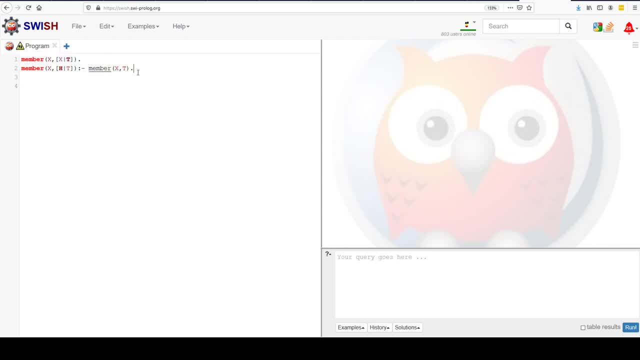 will end up identifying true for every possible word or element that's contained in the list. So let's head over here. let's do. member. let's look for Mia in the list. Yolanda Mia Vincent. actually, you know what? for the first example, we should leave it at the head. so 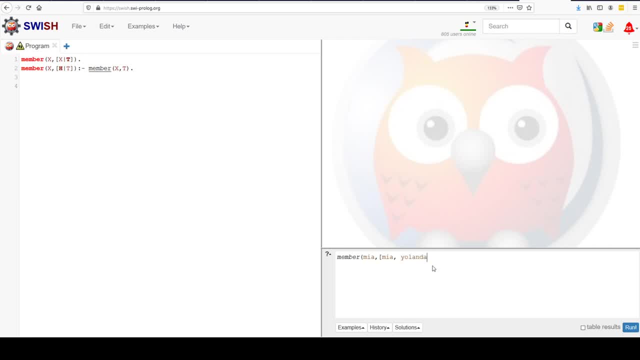 Mia, Yolanda, Vincent and Jules. So we're going to check if Mia is a member of this list. That's the idea of the member predicate: is this element a member of this list? So we got true. we got a couple of singleton variable warnings. I'll talk about those in a second. 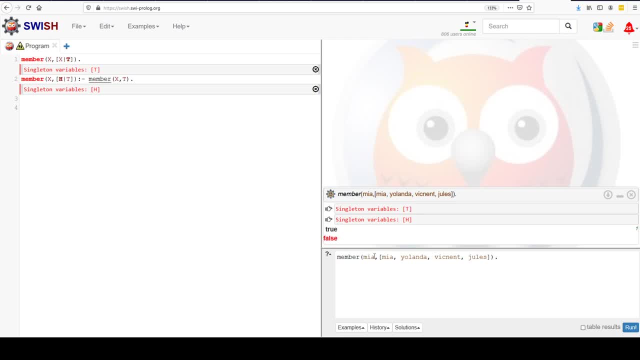 but we got true and then we got a false. So the reason we got true and false is that this: I'll evaluate it to be true. this is the first thing we checked. Mia and the head of this list are the same Mia and Mia. but once we find one true, we keep searching. 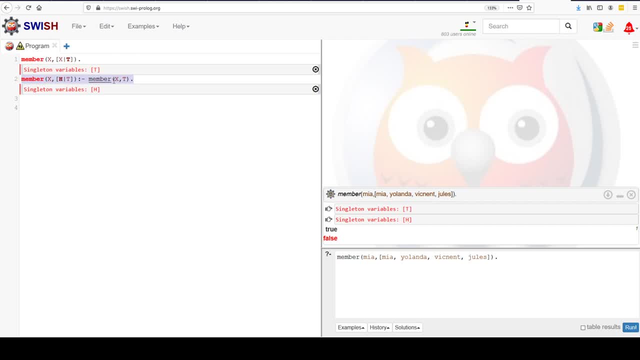 so we recursively tried this list or this, this predicate, sorry, and it recursively called both predicates again, but with the tail of the list. So in other words, the prologue keeps running through all the options. and so we first compared Mia and Mia and found: 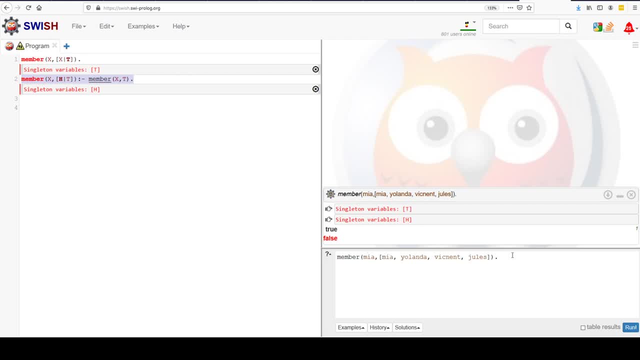 it to be true, but then we iterated through the rest of the list and looked for more Mias, and there weren't any more. One thing that's interesting about this process is that it is that if we had a second Mia in the list, we're going to get true, and then true again. 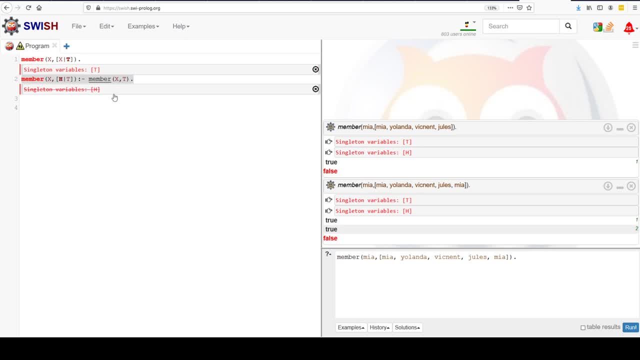 and then false. So we're going to find the first Mia and then recursively iterate through the whole list, and the way that this ends up stopping, the way that we end up getting a false, is that every predicate requires splitting the list into a head and a tail. 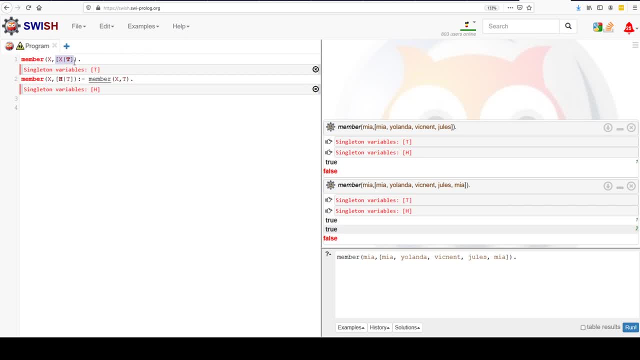 so once we have an empty list, both of these were guaranteed to evaluate to be false, and so we'd never actually call the recursive call eventually, once we have a list, that is split into a head and a tail. So let's take a really let's take a shorter and simpler. 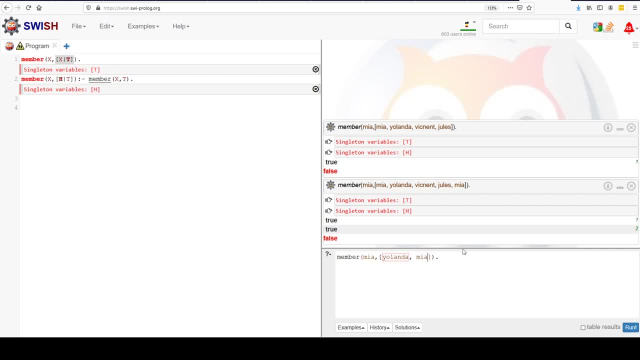 example here, Just Yolanda and Mia. I'll run it. we're going to get a true and then a false and let's walk through the recursive steps here. So first we call: we check member with Mia, and then Yolanda and Mia. So the first thing we do is we check member x comma, x comma. 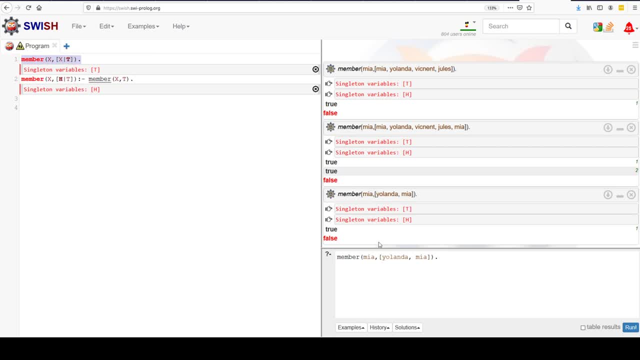 and then we split our list into a head and a tail. So the head of the list is Yolanda, x is Mia. these two do not unify, so we're going to move down to the second predicate here. So we're going to take x, which is going to be Mia. it's our only option and we're. 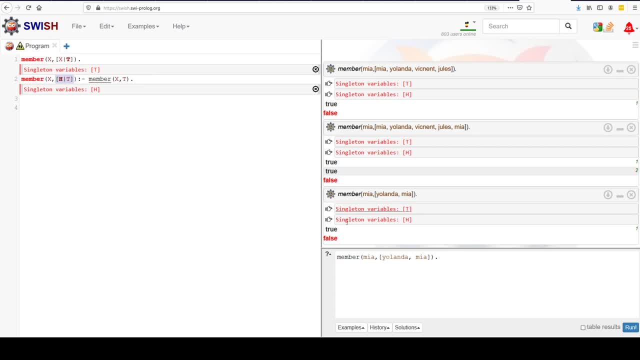 going to check our list, which is Yolanda, and Mia split it into a head and a tail. head is Yolanda, now Yolanda. here is going to be h. h doesn't have to unify with anything, so that's fine. 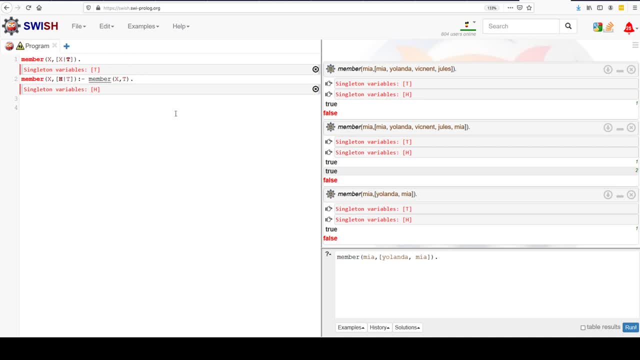 The tail is going to be Mia as a list, Right? so first iteration we have: h is Yolanda, x equals Mia and t equals Mia, but as a list. And so we call member again for our second iteration And we're going to pass in Mia as x and Mia as a list as the tail here. So we're going. 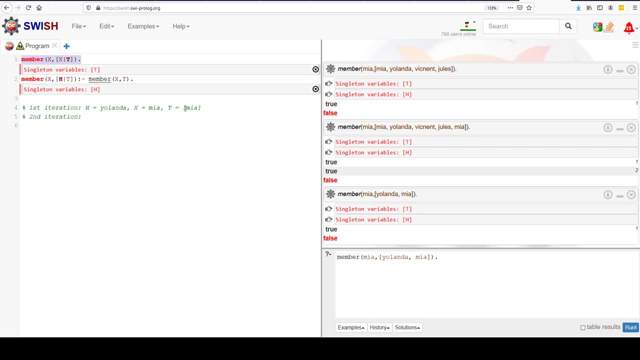 to come to our first member here- and x and x are the same. If we split this list into a head and a tail, we're going to get that x equals Mia and t equals empty list and x equals Mia. So these unify. this is where we got our first true. Now we have to continue. 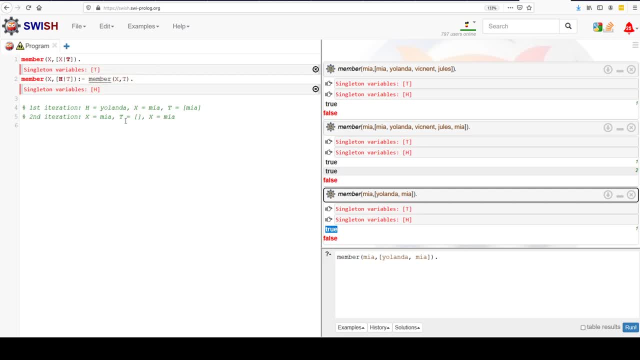 running, So we do one more pass down here. In this version, h is Mia. We've changed our variables. x is still Mia from the thing we're looking for. h is Mia for the head of the list, which is still fine, And then t is the tail, which is empty, And so we call member. 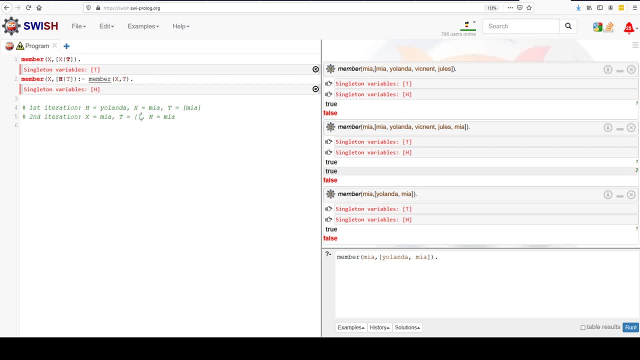 again And when we call member again, t is an empty list. So that means that when we even try to run these predicates where we split a list into a head and a tail, if you try to split an empty list into a head and a tail, it's always false. So neither of these. 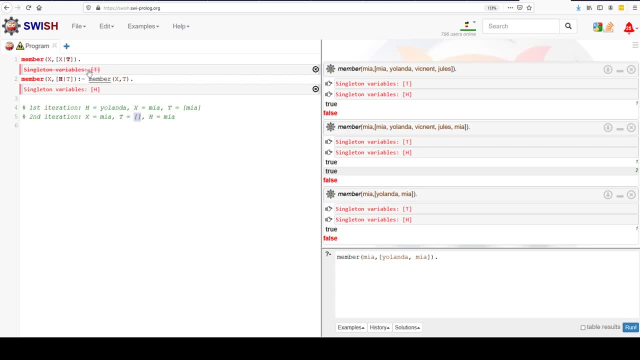 run and so we get false and we're done. So this will work to find any member you want to in a list. The last thing I wanted to highlight is that we don't care about the tail in this particular predicate. We care about it here, but not here, And so an anonymous variable. 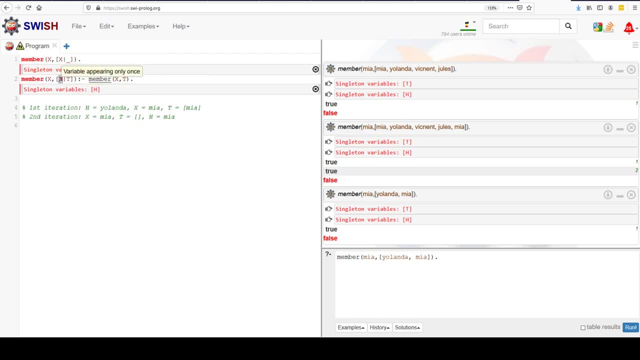 is better here And in this predicate. we don't care what's at the head of the list, so an anonymous variable works there. So this is probably the best way to run this And that's how we really write it. Hopefully that makes sense. We'll do a couple more examples. 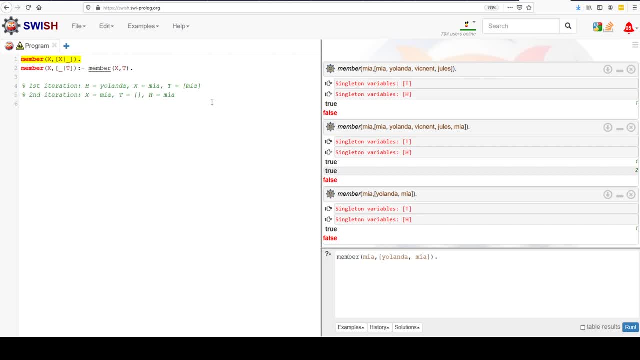 here with a couple different ways that we can write these expressions. But as we go through, if you kind of run through iterations of this, you'll see that you'll be able to find every item that is a member of the list. And then, I guess, the last example I was trying. 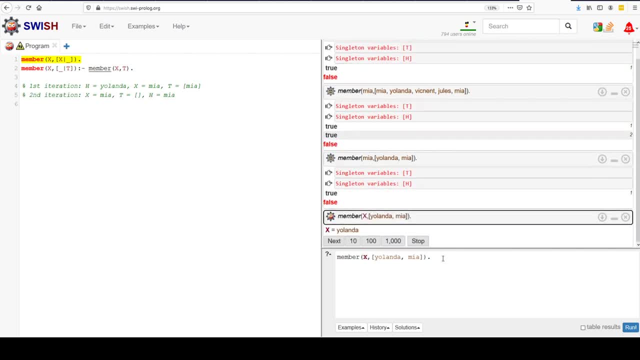 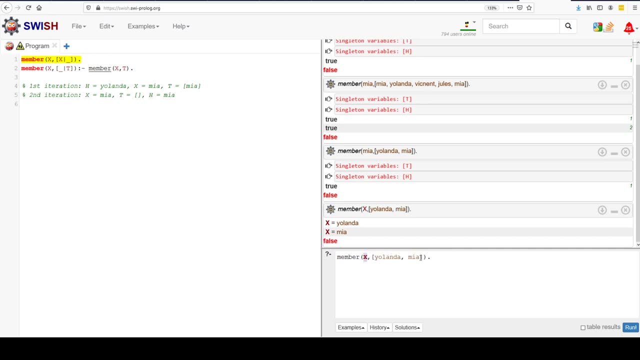 to wrap up, but I forgot. I wanted to do one more thing. If you set a variable like x as the thing you're looking for, it will find each element of the list one at a time. So if you have a five element list as we iterate through, it's going to find every. 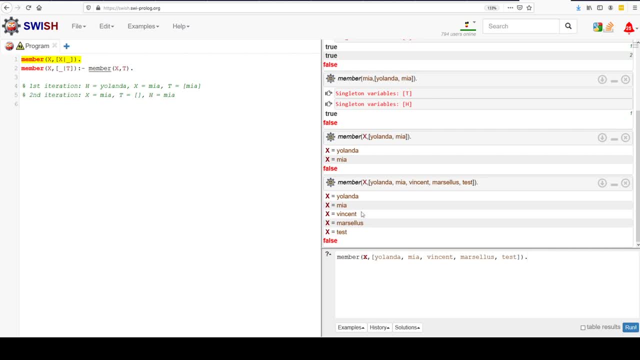 possible x. that is in the list. So this is a good thing to go back and look at as well- What happens if you put variables in, And so hopefully this makes sense. We'll do a few more examples. Really, the best way to learn Prolog is to watch a few examples and then. 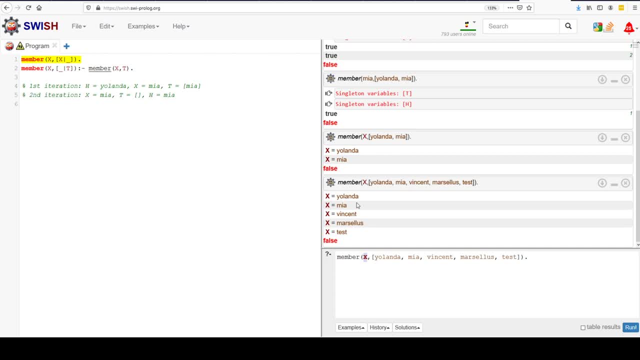 try a few problems where you can look up the solution. You'll see a 99 Prolog problem set in Moodle that you could look at. So take a shot at that. But we'll do a couple more examples before I turn you loose. See you next time.